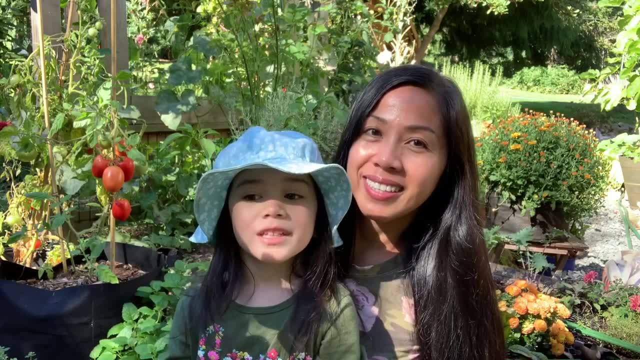 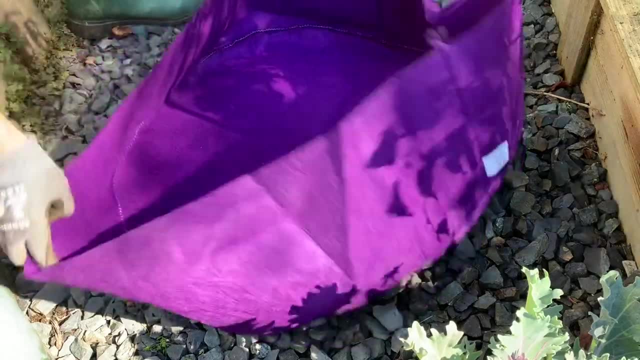 plant. Go ahead, We're going to plant a dinosaur garden. Okay, All right, guys, let's play in the dirt. So I'm going to open it up and get it set up, so that way we can put the dirt in there. 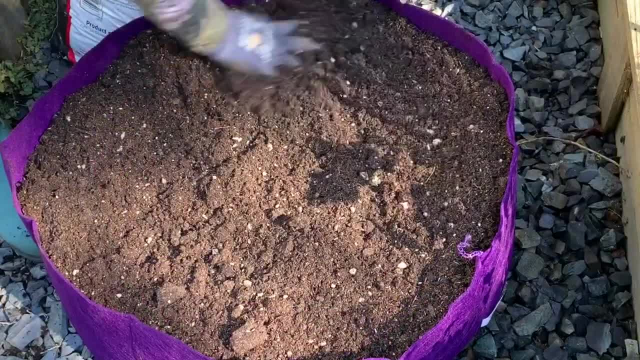 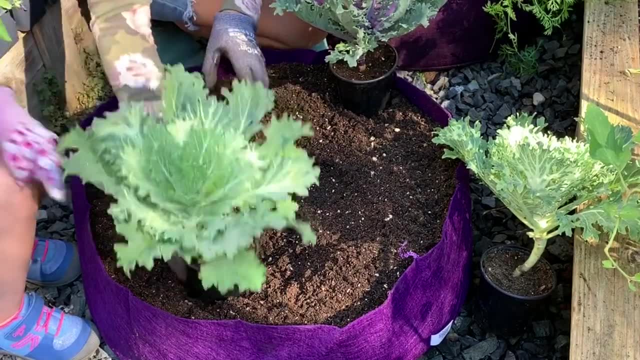 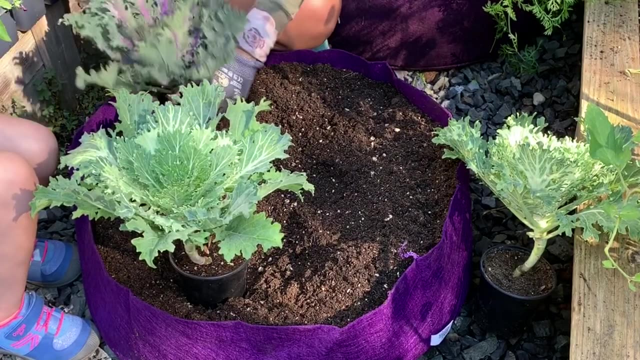 So let's go ahead and put these down where you want to plant them, okay. Where do you want this one? Uh there, Okay, perfect. And the purple one right here? Right here, Okay. And how about the other green one? Well, I'm going to dig a hole, Okay. 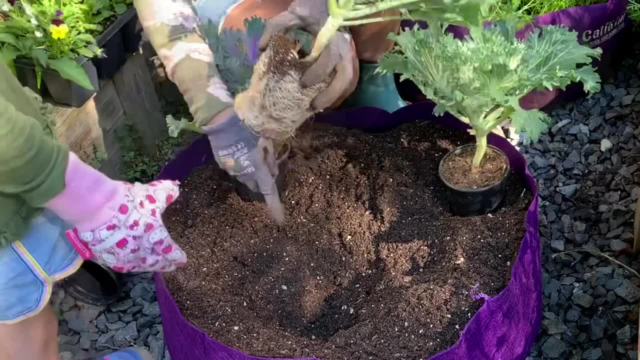 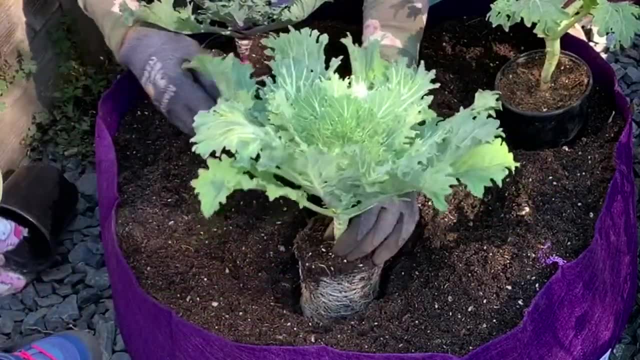 Pinch the roots a little bit- okay, Good job, And go ahead and place it in the hole. I'm going to use two hands There you go, So I'll hold it for you and then go ahead and put the dirt around it. Okay, Good job, honey. 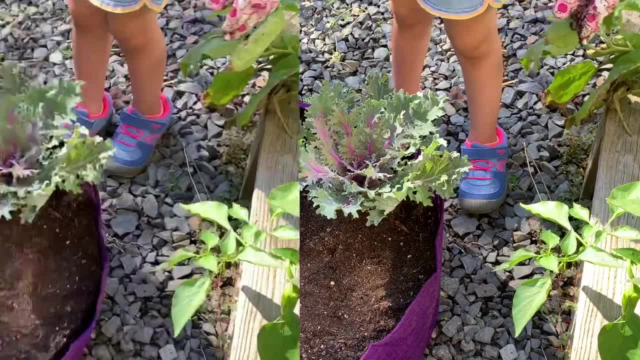 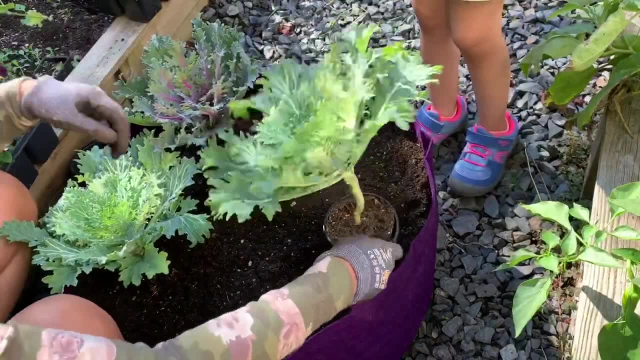 Good job, Woo-hoo, you did it. Spin it around, Spin it around, Rotate this. So now you can reach that side. okay, So I think you want to plant it right here. Oh, and I'll do this, I'll put my finger in. 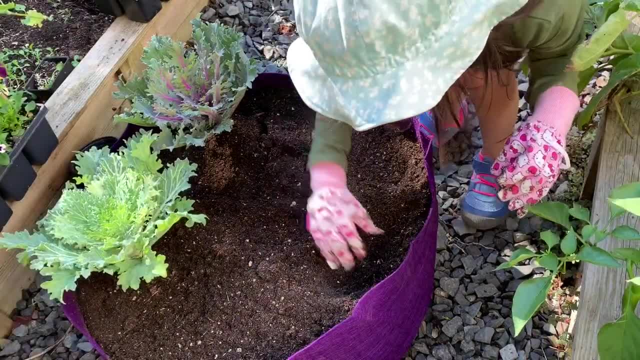 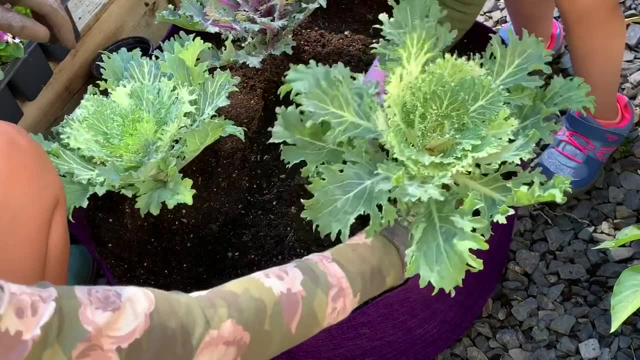 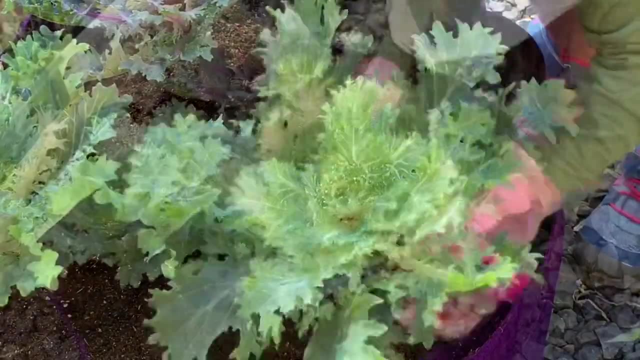 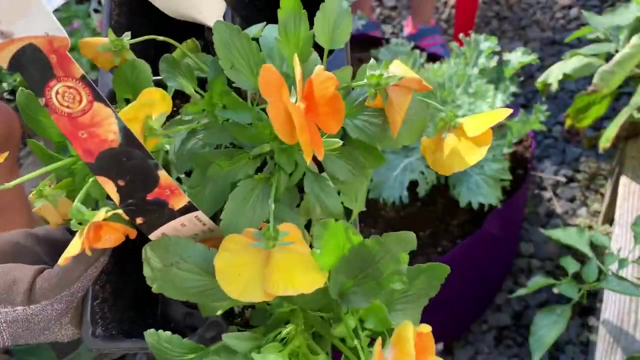 the dirt. Yes, go ahead, honey, And backfill Ready, I'll hold it for you so you can pull the dirt back in. We're also going to plant these yellow-orange pansies, which will look really nice with a purple pot, So it's a great contrast. 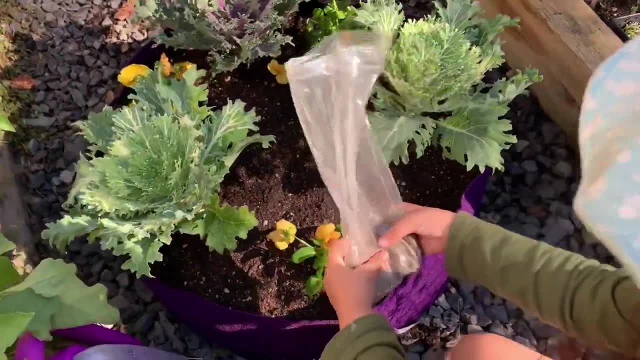 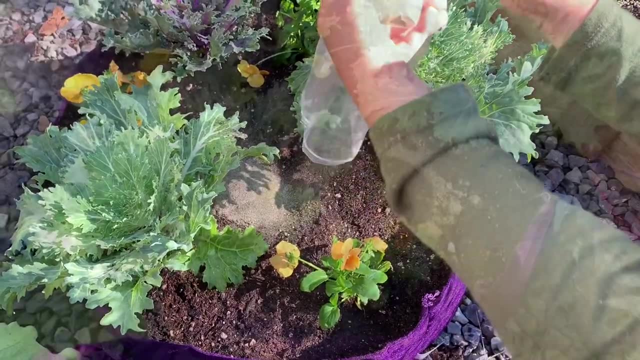 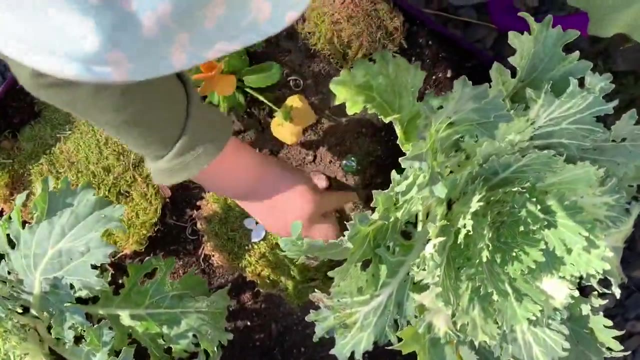 So now we're going to decorate her dinosaur garden. So first she wants to pour some sand. Go ahead, honey, So you can spread that out. We'll also be placing some moss and some rocks. Some rocks- Where can I put it On here? Anywhere, honey.